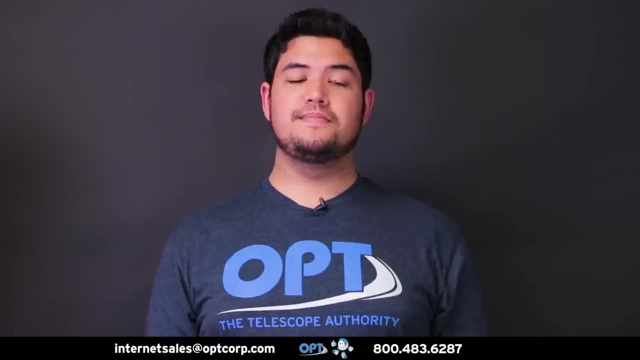 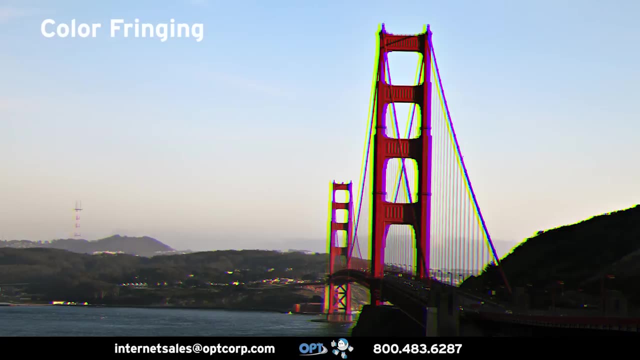 considerations you'll want to keep in mind when it comes to refractors. Depending on the type of lenses used for the optics, you may encounter visible color fringing at high magnifications, Also known as chromatic aberration. color fringing is when various colored wavelengths 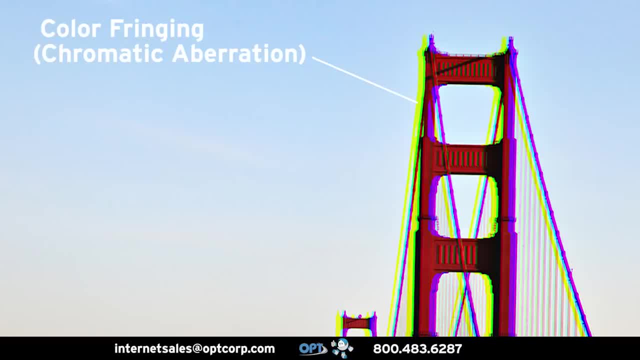 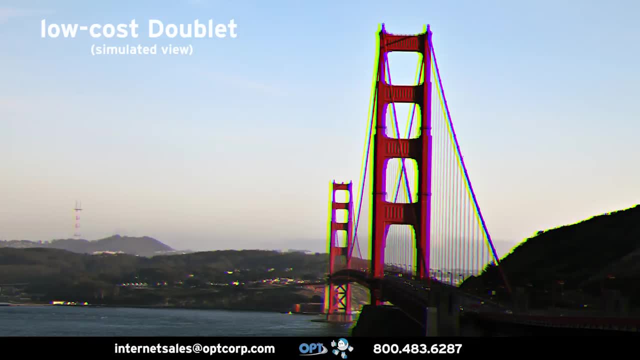 of light get split from each other and arrive at slightly different angles than the other angles, showing up as an image with distinct coloration at the edges. Most low-cost refractors are doublets, which may have color fringing, whereas triplet refractors are designed to. 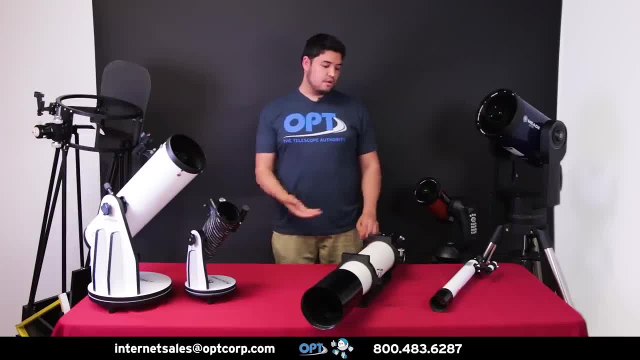 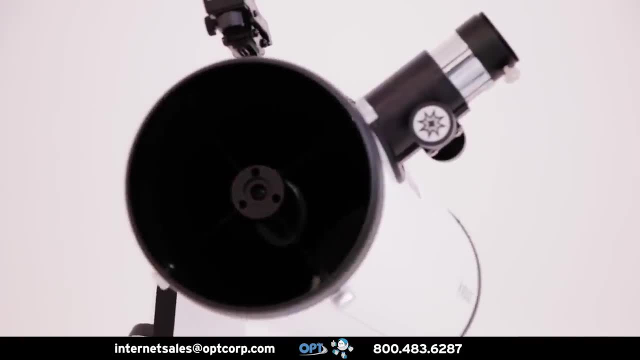 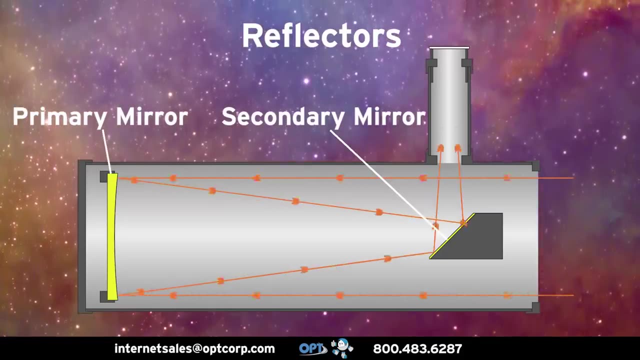 eliminate this issue. Still, whether a doublet or a triplet, refractors are solid, sturdy and require very little maintenance. Next, we will discuss reflectors. Their use of mirrors causes light to reflect at various angles within the optical tube, which extends the 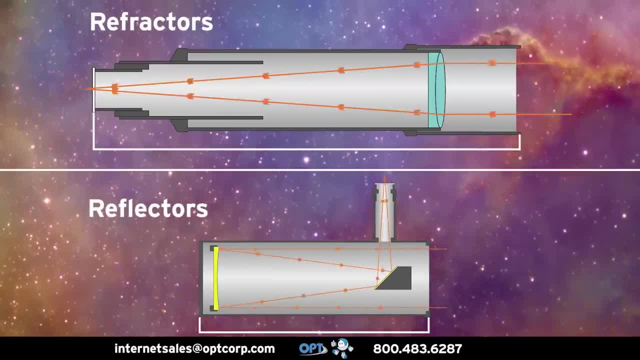 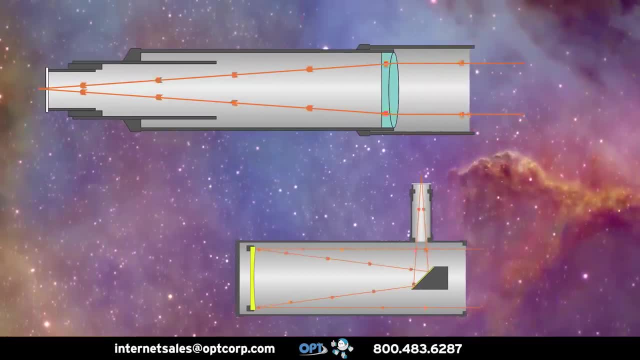 overall light path. This often causes reflectors to be shorter than refractors of the same aperture, as the light doesn't need to flow in a straight line to move the same distance. Since manufacturing large mirrors is often cheaper than manufacturing large lenses, it is fairly common for reflectors 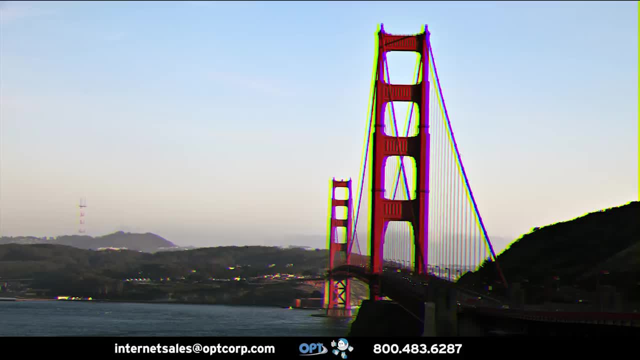 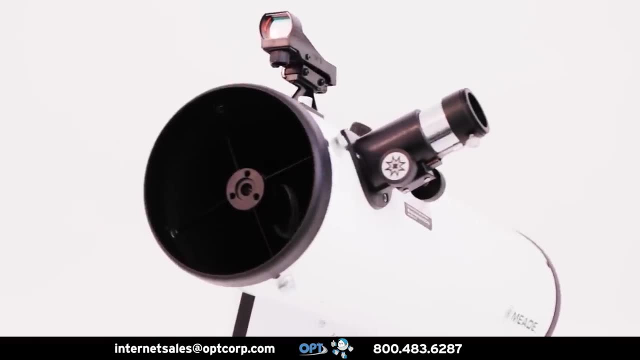 to be much less expensive than refractors. Additionally, reflectors are not susceptible to color fringing in the same way that doublet refractors are. If you're looking for a lot of bang for your buck in terms of aperture, reflectors are a great way to go. This is. 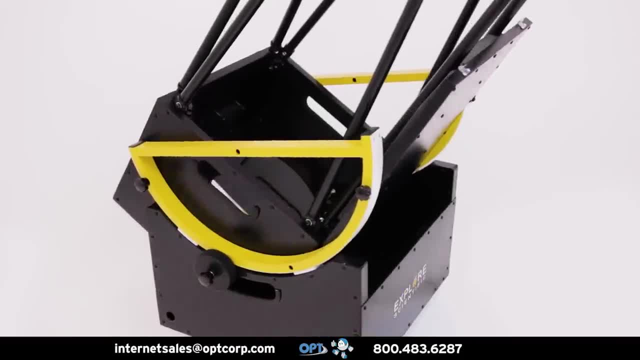 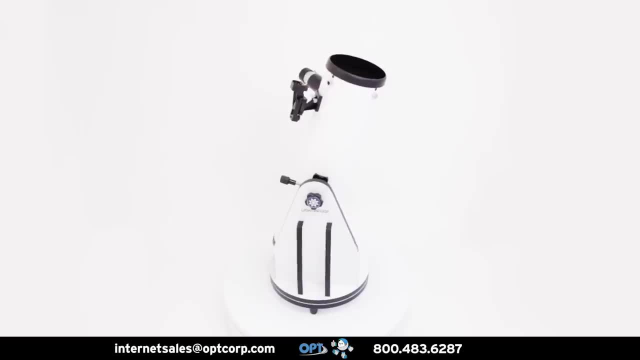 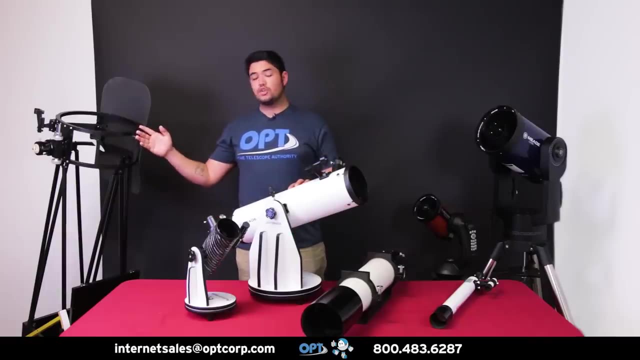 especially true for Dobsonians, which come with their own easy-to-use rocker box. mount Reflectors can be of great value with many conveniences. They can also come in a variety of sizes and can get quite large. Because of this, purchasing the largest reflector you can get is a great 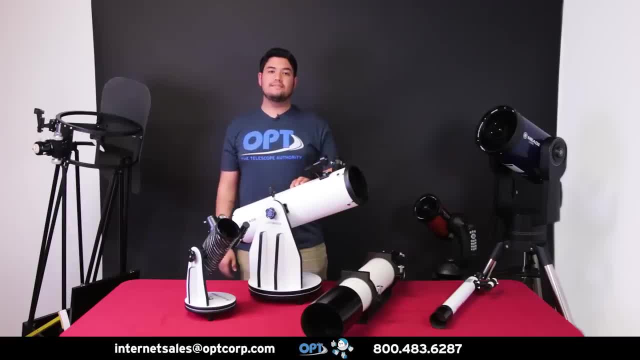 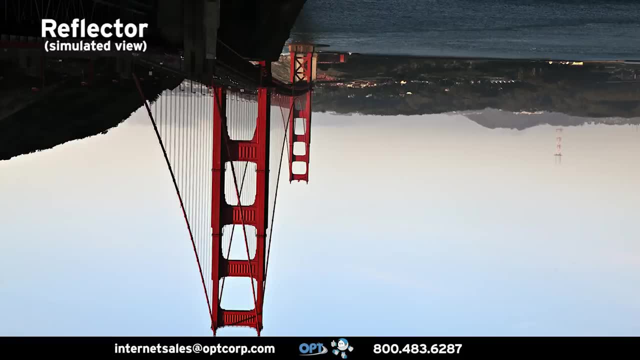 way to get a low-cost, large aperture telescope. Another consideration is that, by default, the image you see through the reflector's eyepiece will be upside down. For this reason, you'll want to use your scope's finder to line it up with the objects you want to. 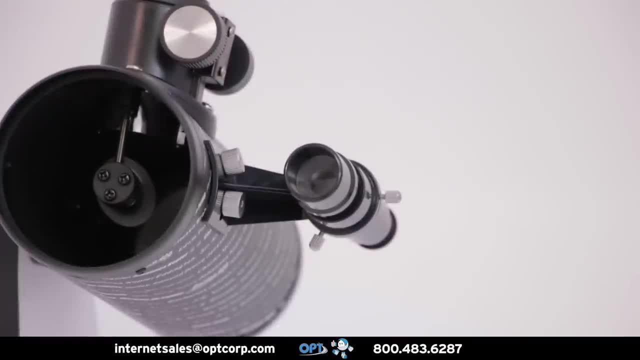 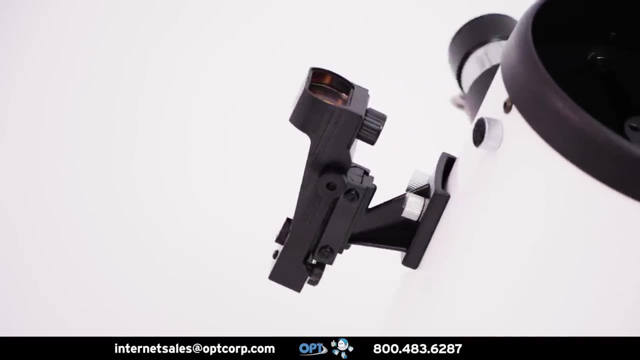 see before looking through the eyepiece. Most modern reflecting telescopes come with a finder scope or a red dot finder, so you won't have to make an additional purchase to acquire this. Lastly, a reflector will sometimes require a process called collimation. 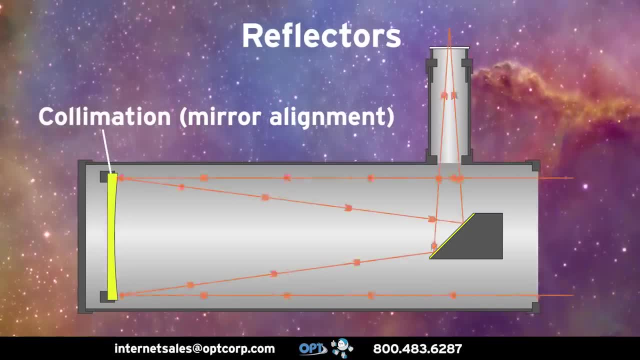 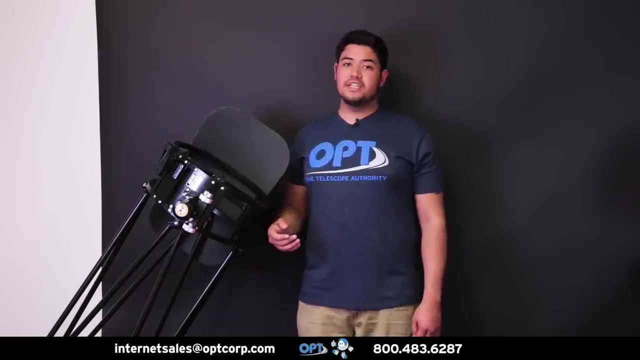 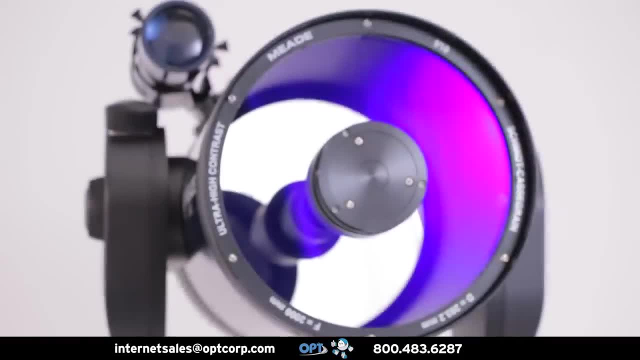 far away from you or objects that are far away from you or objects that are farther than you. You should also be careful with the way you sleep, but also remember to limit the light source and remain on your own bed. 3- Last but not least, we will discuss Catadioptric or compound telescopes, As previously. 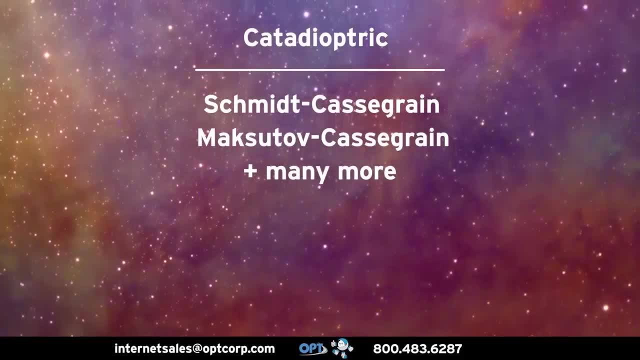 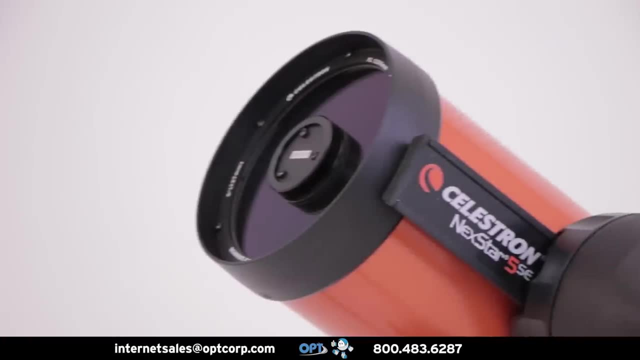 touched upon. there are many variations on this design, Regardless of the specific build. Catadioptrics combine the optical benefits of both lenses and mirrors into a compact, convenient package. This makes them more portable than either refractors or reflectors of the. 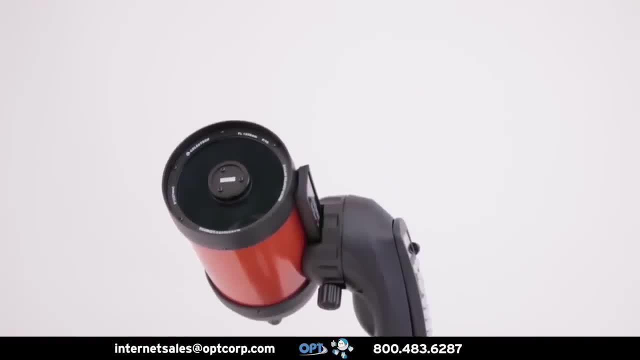 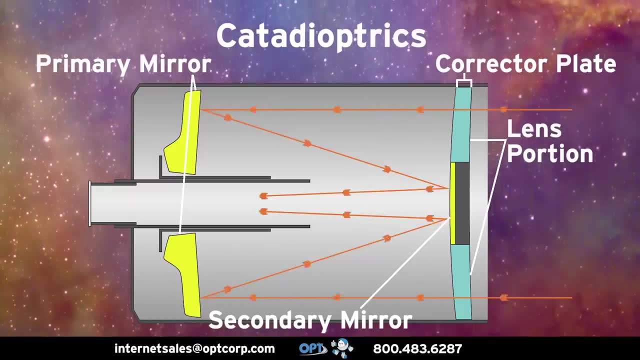 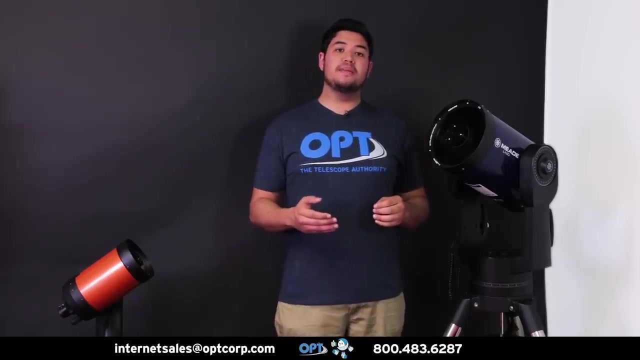 same aperture. This is made possible by the corrector plate that folds the light pack path and the curved secondary mirror that magnifies the light internally. Since it uses mirrors like a reflecting telescope, catadioptric telescopes still require collimation. 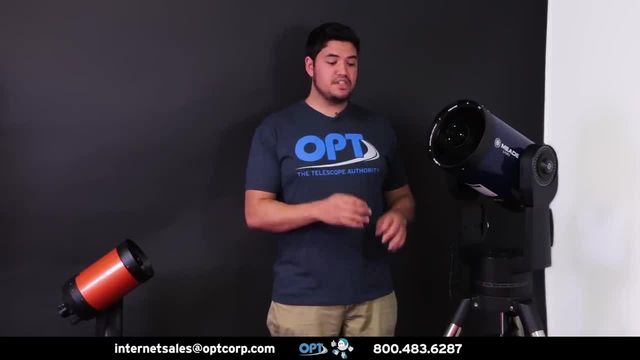 Unlike reflecting scopes, catadioptrics require this collimation far less frequently. A well-maintained and kept catadioptric scope can maintain collimation for years. The catadioptric's small size and portability gives them a convenience not found in reflectors. 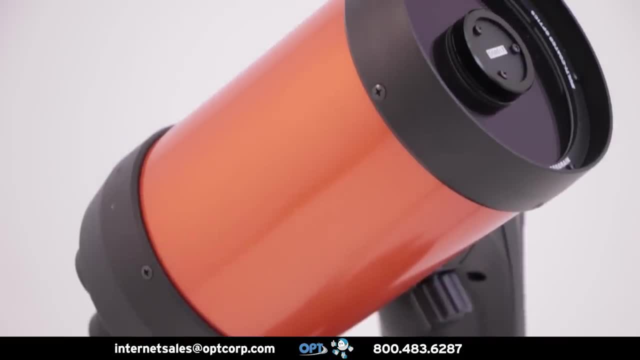 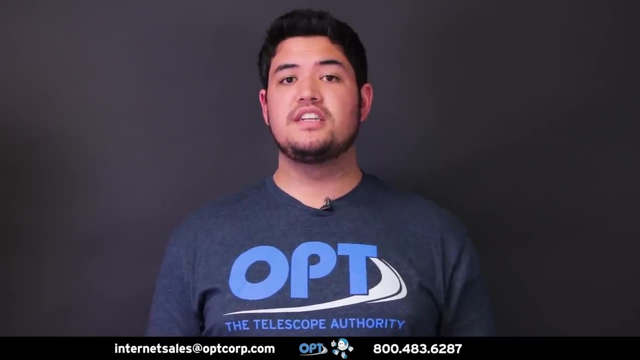 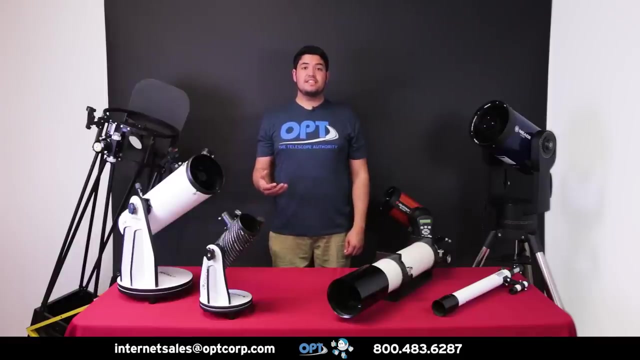 of the same class, making them a great investment for both beginners and experienced astronomers alike. So which scope is right for you? Well, in most cases, you're going to want the largest scope that you can reasonably afford and carry. However, you might have specific needs that could make one telescope type better for you. 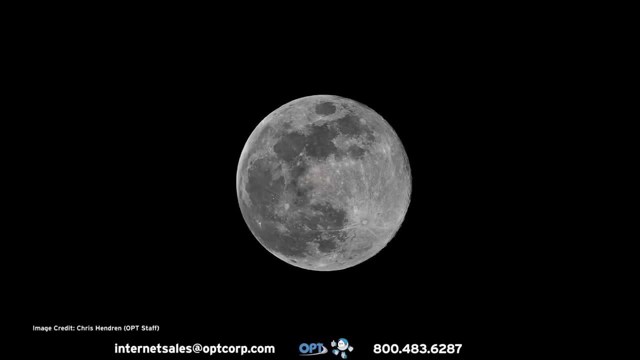 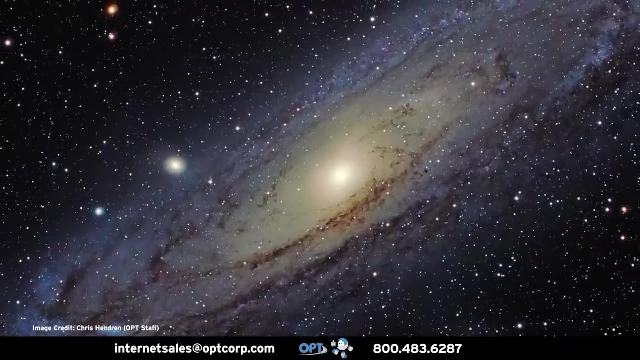 than another. If you're on a budget and just want to observe the moon and the various nearby planets, a small scope like a basic refractor is a great value. If you want to do deep sky observing of distant galaxies and nebulae, you may want to consider 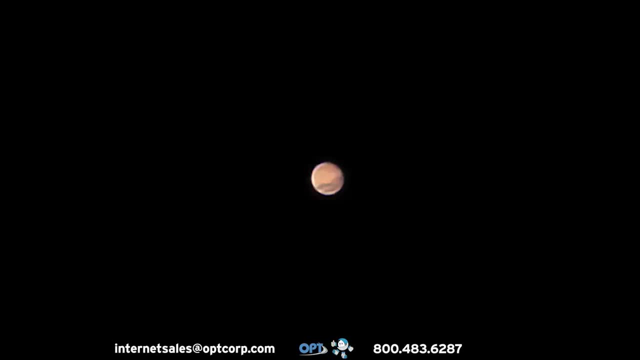 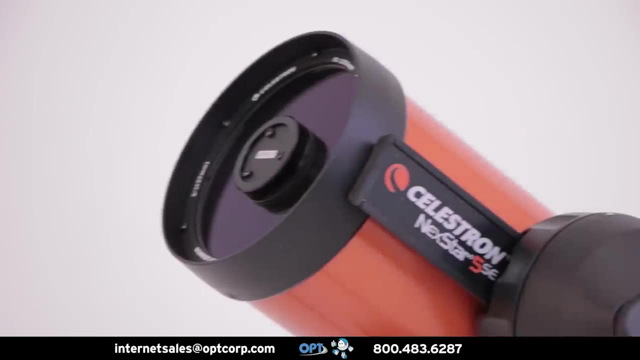 picking up a large reflector. If you want a high degree of flexibility in what you observe, a Schmidt-Cassegrain or other compound telescope will give you a lot of options for your viewing experience. Hopefully we've cleared up some of the confusion regarding the basic telescope types available.